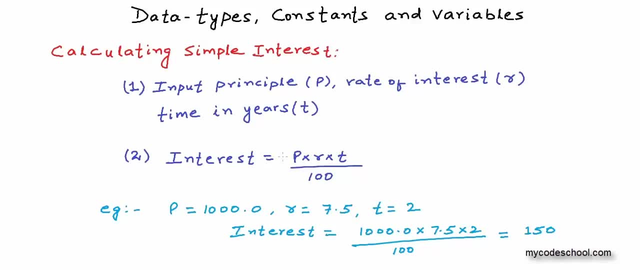 If you look at this expression here- p into r into t, upon hundred p, r and t- here are variables. Variables by general definition are things that can change In this expression. p, r and t can be anything. Hundred in denominator is a constant. A constant is something that won't change. Hundred is a hundred in any part of the world. We have concept of constants and variables in programming also. You can use this concept in programming as well. 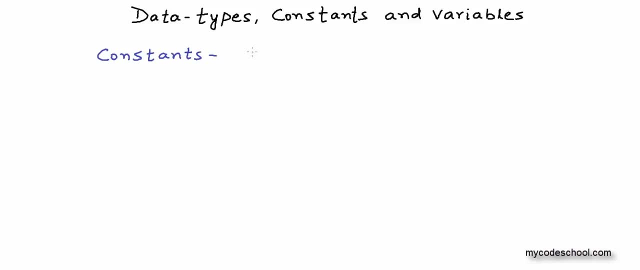 You can think of constants as values of different types that you can write directly in your code, in your program: An integer, a real number, a character or a sequence of characters that we call a string in programming- Names, words, phrases and sentences in a program- all of these are strings. If we use values for these different types directly in our code, then we call them constants. There are defined set of rules to create constants of different types. 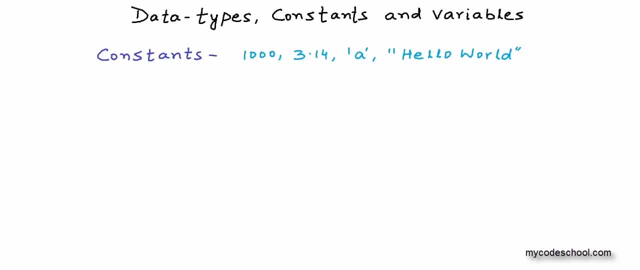 And sometimes a constant can also have a name or identifier. I will talk about these concepts in a while. We can think of a variable as a unique name or identifier for a section of computer's memory where we can fill in some data. So if p and q are two variables in my program, you can imagine them in the memory like how I am showing here. p is only a name for this section of the memory. 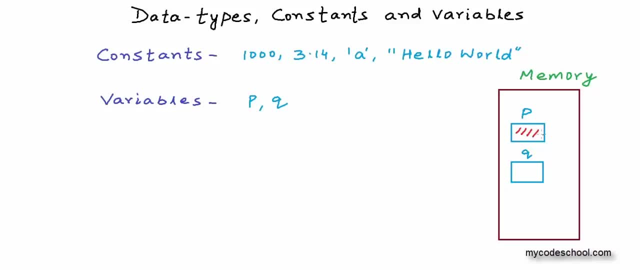 And using the identifier, we can call it a string. If we use the identifier p in our program, we can store some data here in this section of the memory. Basically, we can read and write to this section of the memory. Similarly, q is another variable that is identifier for this part of the memory. Once again, using the identifier q, we can read and write to this part of the memory. 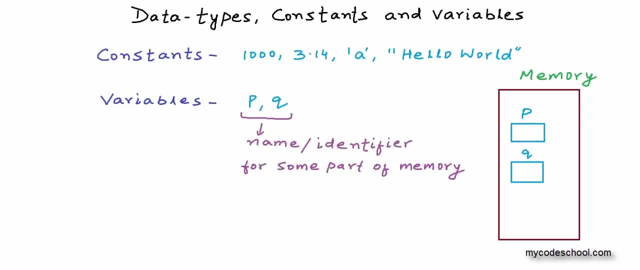 In programming. quite often we use this term identifier for name. That's why I am saying identifier a lot of times. Once again, to create and work with variables, we need to follow the rules of language. Constants and variables in a program are means to store and represent data. 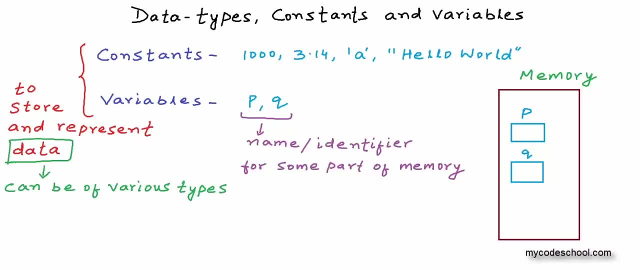 Now data can be of various types. Different types of data are represented differently. We saw some of the types while writing these constants. Data can be a number, sometimes an integer, sometimes a real number. Data can be a word, phrase or sentence, And then there can be all kinds of complex forms of data. 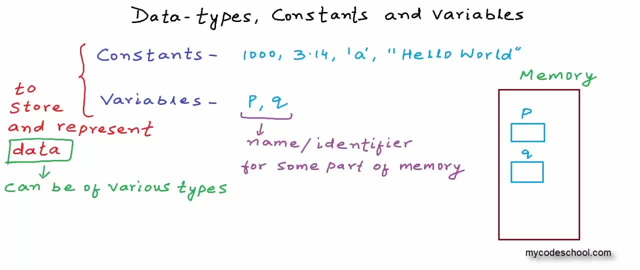 And the kind of operation that you perform on different types is different. Moreover, any data that has to be stored in computer's memory has to be binary, has to be a pattern of ones and zeros. Any data from the real world first has to be encoded or converted to binary, And then it can be stored in computer's memory. 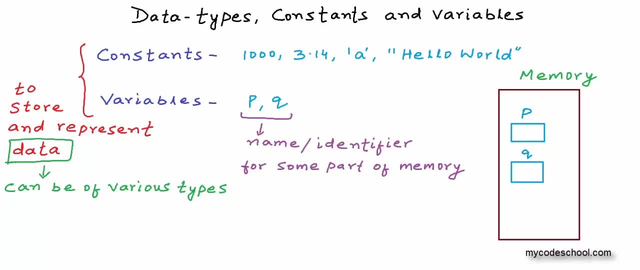 So there will be different encoding mechanisms for different types of data. We will talk about this in detail later. For now, just understand that different types of data are stored, stored differently in computer's memory. A constant or variable in a program must be: 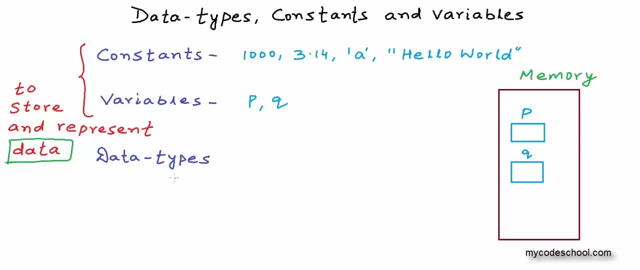 of a defined data type. A programming language gives us definition for some basic data types that we call primitive types, and then the language gives us tools to create complex types or composite types using primitive types. So primitive types are already defined in the language, and composite types need to be defined by us. In our initial lessons, we 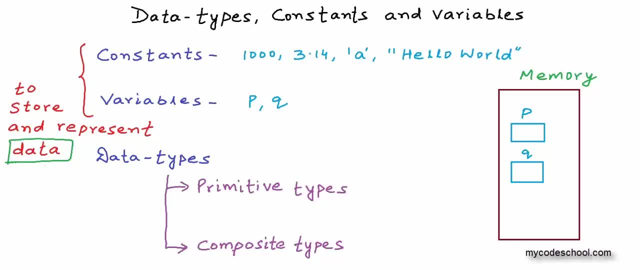 will mostly be talking about and working with primitive types. Most famous primitive data types are int for integer, char for character, float for real number, and there is another one for real numbers. It's called double. Int, char, float, double. all of these are 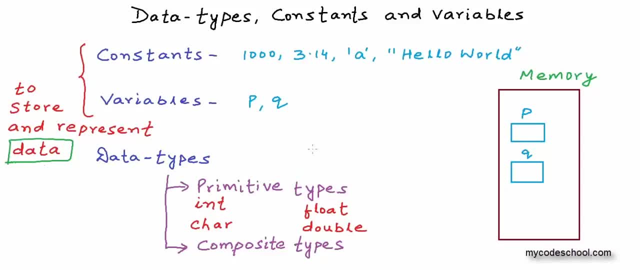 keywords. Keywords are reserved words that are always used in a program for a specific purpose, with a specific meaning. So these keywords will always be used to mark the data type of something. There are some other primitive types in C. We will talk about them later. There is one more building. 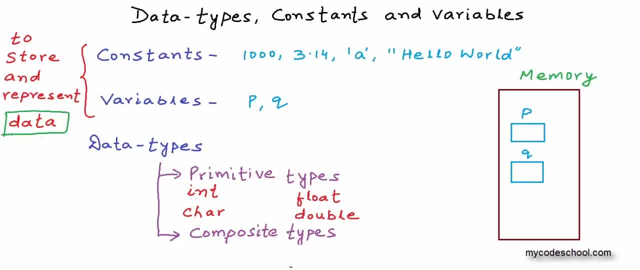 block that we need to know about and then we can go ahead and write some programs to perform some real computations. We must know about operators. Constants and variables are means to store and represent data. Operators specify what to do with data, what operation to perform with data. I will list down some of the operators. Operators are also of different. 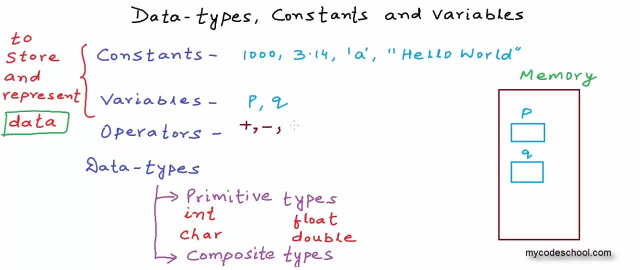 types. We have arithmetic operators: plus, minus for addition and subtraction, asterisk for multiplication, backslash for division and percentile sign for modulus operation. These are arithmetic operators. A single equal to sign is called an assignment operator. It is used to assign value to a. 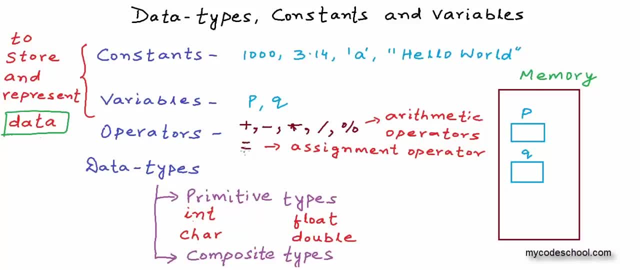 variable and we have operators that we call relational and logical operators. 2 equal to sign is for equality operator. if you want to compare two values for equality, you use 2 equal to signs. This is a logical operator. and then we have operators like less than. 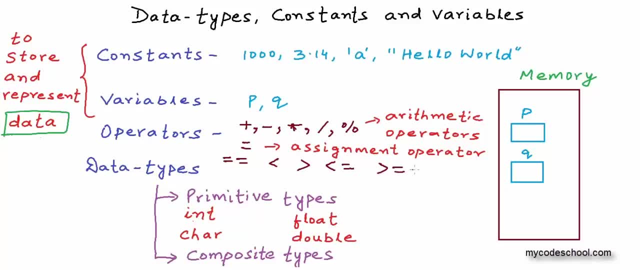 greater than less than or equal to greater than or equal to greater than or equal to greater, equal to greater than or equal to. These operators are called relational and logical operators. We will get to know these operators when we will use them in a real program Constants. 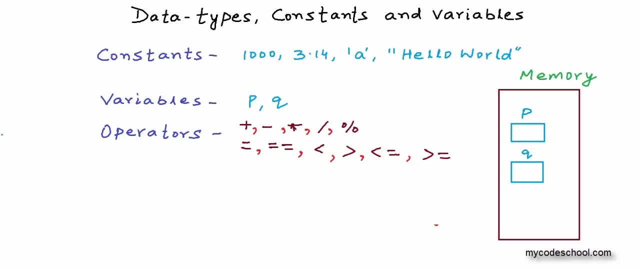 variables and operators are combined together to create mathematical and logical expressions that would evaluate to something. For example, let's assume that p and q are variables of type integer, then p plus q will evaluate to the sum of values stored in p and q. p. 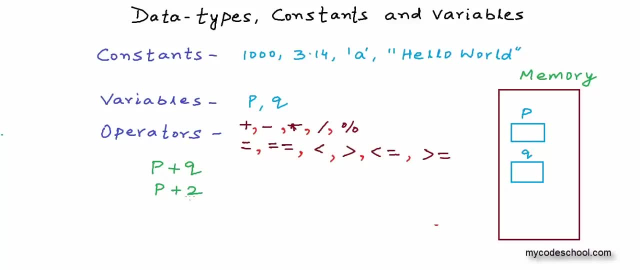 plus 2 will evaluate to the value stored in p plus 2.. Now, 2 is a constant. here, 2 is a constant of type integer, and we can have complex expressions also, like this one, to calculate simple interest. Let's now see how we can use these building blocks in a real 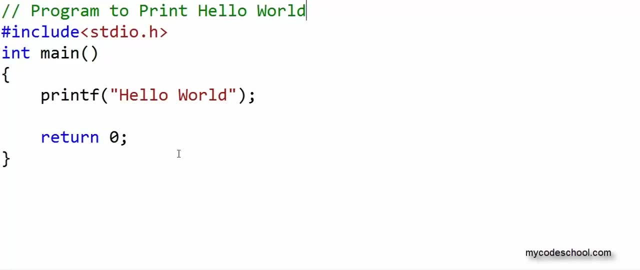 program. I will start where I had left. This is the program to print hello world that we had written earlier. As we had discussed, a C program is organized in entities that we call functions. We must always have a function named main in our program. 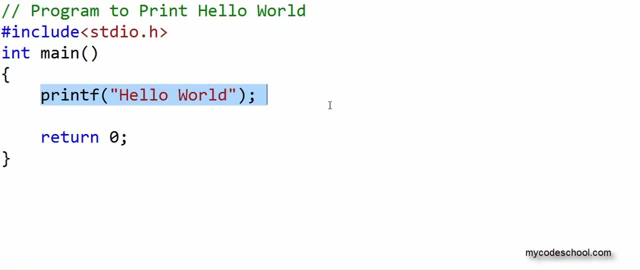 Program execution always starts with first statement in main function. There are some functions that are pre-implemented and available to us in what we call language libraries. To use those functions we need to reference the language library to which they belong. This statement here. 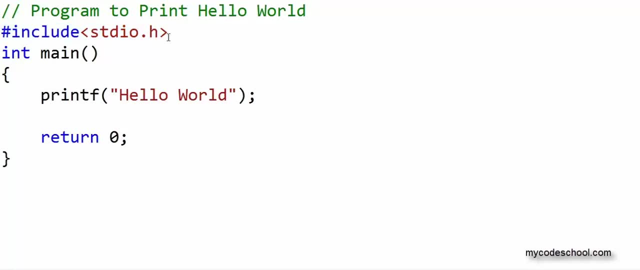 include stdioh is referencing the library. stdioh Printf function that we are using here is part of this library. The first line that I have written here is a comment in my program. Comment in a program is text that is ignored by the compiler. It is not considered. 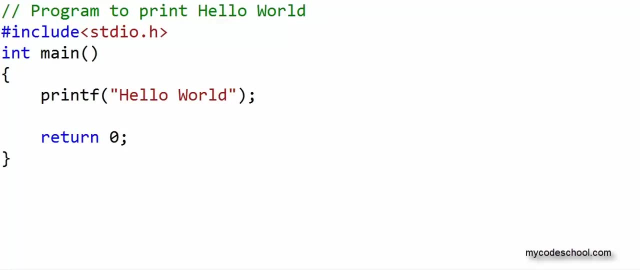 for execution. You write a comment in a program for things like mentioning the name of author of the program, or for describing problem statement, Or for explaining some part of your code, all in natural language. There are two ways to write comment. If you write something starting two forward slashes, then everything starting. 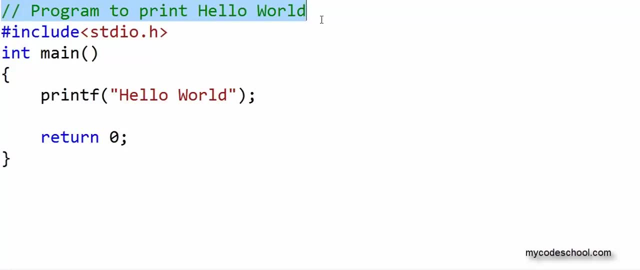 the slashes till the end of that line is a comment. in your program You can begin a comment after a see statement. also, Another way to write a comment is start with forward slash and then put an asterisk sign and then everything after that is a comment, unless you close the comment. 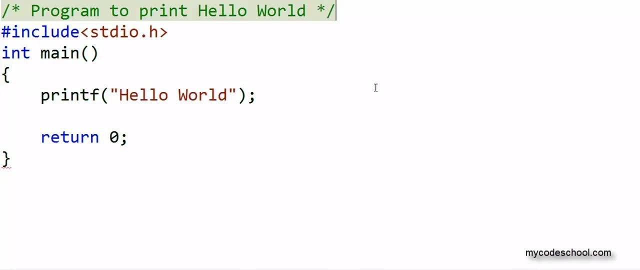 with another asterisk sign and then a forward slash In closure. asterisks would come first. Using this method, you can write a comment in multiple lines, Okay. so what I'm going to do now is I'm going to write a comment using constants and variables, So we are going to learn how to create. 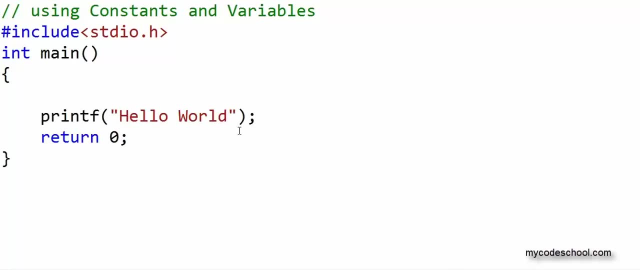 constants and variables in a program. I'm going to leave this printf statement as it is for now. To use a variable in a program, we first need to declare it. To declare a variable, you write a statement like data, type, space, variable name, A. C statement must always end with a semicolon. 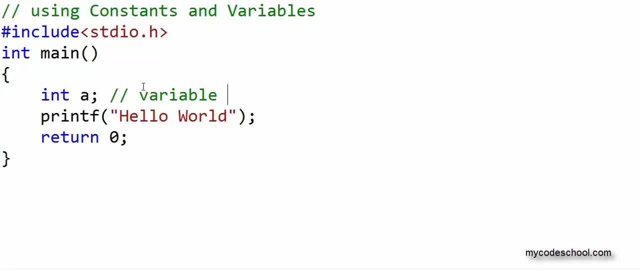 This statement is a variable declaration. We have declared an integer variable, a variable of type integer named a. Basically, what we have done is we have reserved some space in the memory to store an integer and we can read and write to this memory using this variable name or identifier. 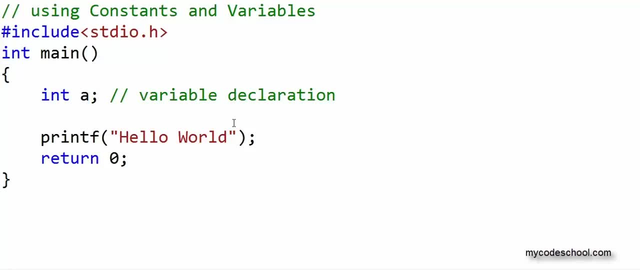 a To fill in some value in this memory or this variable, and we can fill in only integer, because this is a variable of type integer. We can write a statement like a equal, some constant and a semicolon to end the statement, Filling in some data. 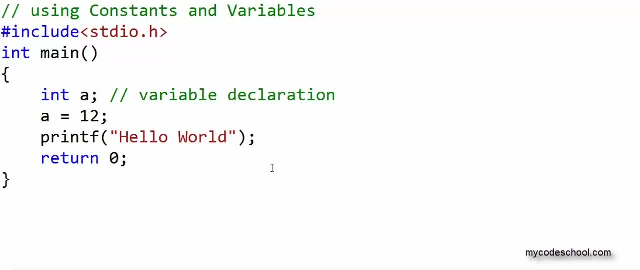 initially in a variable is called initializing the variable. This statement, a equal 12, is an initialization. We can declare and initialize a variable in same statement. Instead of writing these two statements, we can write a single statement like int. a equal 12.. So we are. 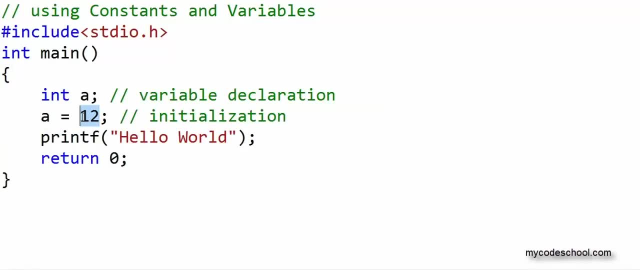 declaring as well as initializing. here, 12 is an integer constant. here, As we had seen, constants of different types are written differently. This hello world here is also a constant. It is a constant of type. string. String is not a primitive data type, It's. 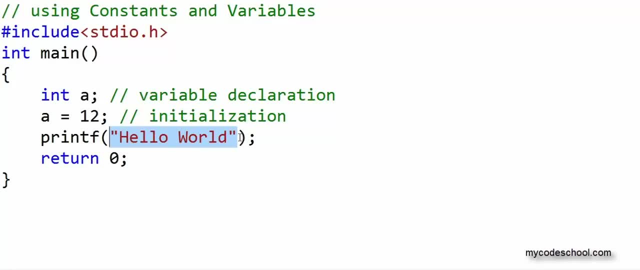 a composite data type. String is a sequence of characters. Character is a primitive data type. A string constant is always written as a sequence of characters within double quotes. This string constant is being passed to printf function as argument. When we pass something to a function, we 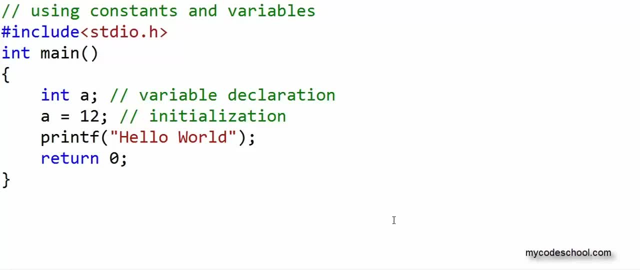 call it an argument to the function, and a function can take more than one argument. It can take arguments. What I'm going to do is I'm going to change this string constant. I'm going to write a equal percent d, So I'm putting this percent sign here and then. 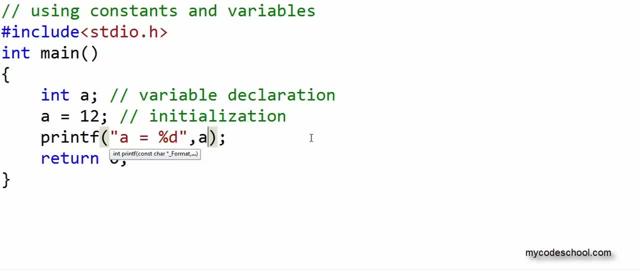 d. and now I'm going to pass one more argument to this function variable a. How many arguments a function will take and what all arguments it will take, depends upon the definition of the function. Printf can take one or more arguments. The first argument must always be: 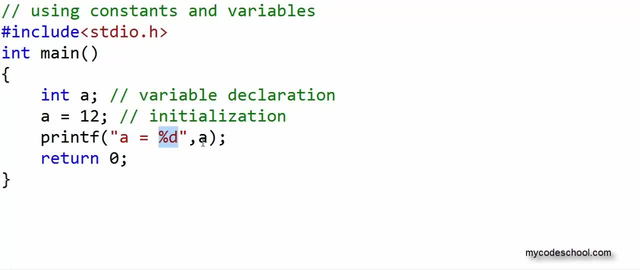 a string constant. If I will put a person d somewhere in this string constant, then printf will expect another argument of type integer and we can pass either a constant or variable of type integer. Now, when printf will print this string, it will replace this person d with the value of this integer. 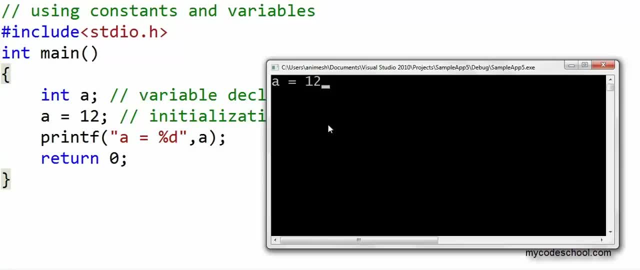 Things will be clear if I will run this program. Upon running the program, this is the output that I'm getting. Printf is printing the string, but it has no value. Now I'm going to as replaced person d with value in variable a. This is called printing a formatted string. 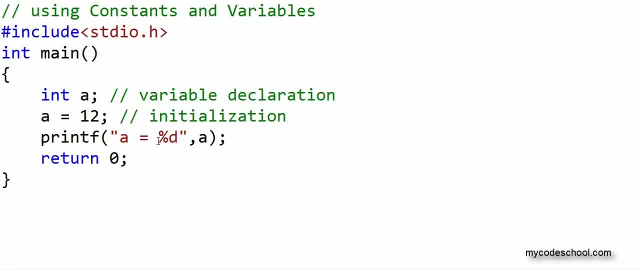 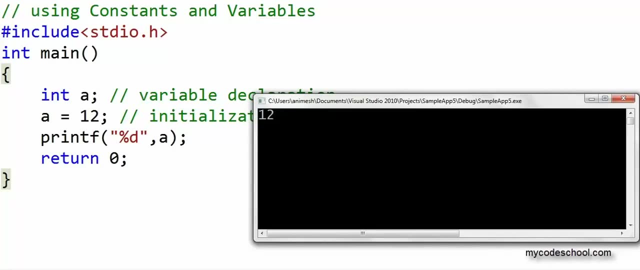 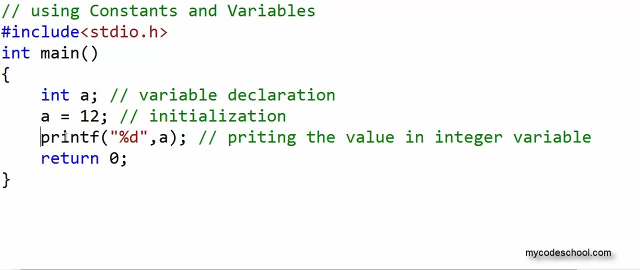 using printf. If we only want to print the value in a and nothing else, we can get rid of this part, and now we are printing only the value in a. Printf is a magical function. it can do a lot of wonderful things. We will see all of that later. For now, this printf: 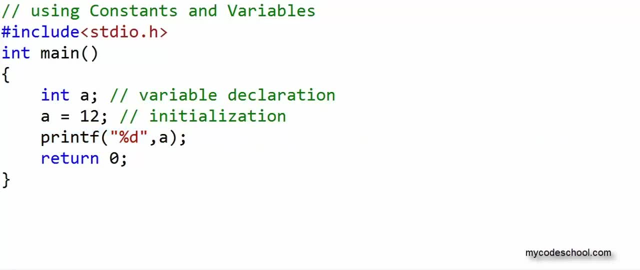 statement is printing the value in integer variable. Okay, so we are declaring and initializing an integer variable and then printing the value in that integer variable. Let's now create some more variables of other types. I want to create a character variable, So I will type in data type- char- And then I need to type in a name. I cannot use the variable. 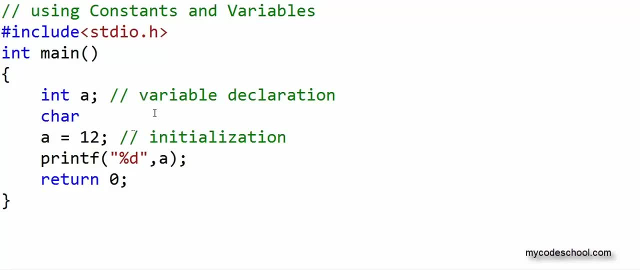 name A. again, two variables within same function cannot have same names. And when I say same small a and capital A are different, You can have a variable name as capital A and and it's fine. Now I can initialize my character variable with a character constant. A character constant is: 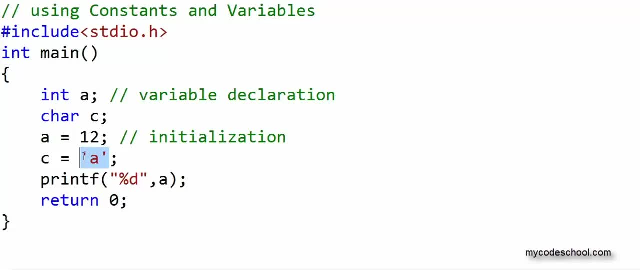 written as a character within single quotes. To print value in character variable: instead of writing percent D, write percent C and then pass the variable C as another argument. Printf will now print the character for you. Now I want to create a variable of type float, So I will be. 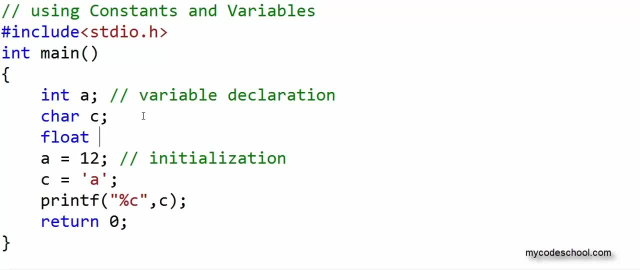 able to store a real number. Name of a variable doesn't always have to be a single character. It can be a set of characters. The rule to create a variable name is that you should start with a letter and then you can have letters, numeric digits and one more possible character underscore. 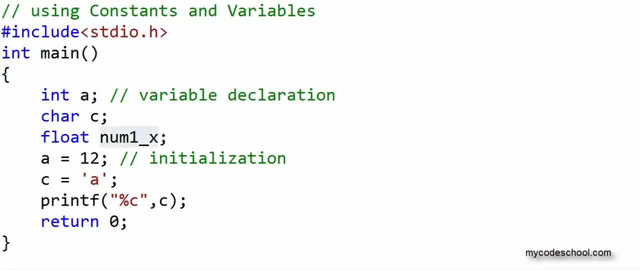 Ideally, a variable name should be something meaningful from real world. And there is one more rule: Your variable name should not be a reserved keyword. in C, Keywords are supposed to be used for specific purpose. in a program like, break is a keyword, So you cannot. 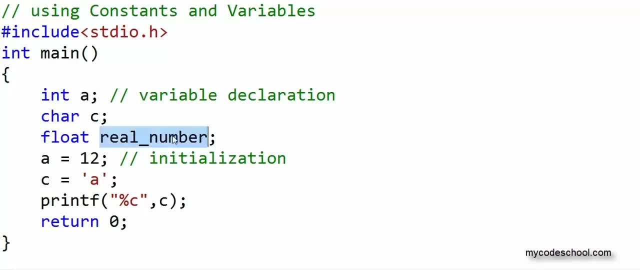 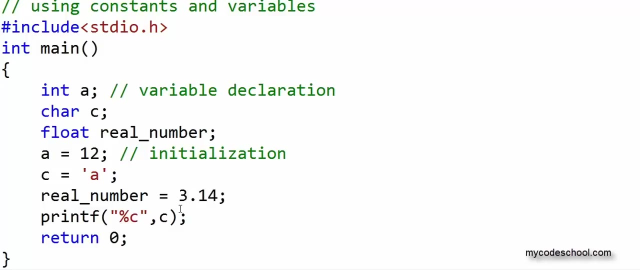 have a variable named break. I will name this variable real underscore number. There can be no space in a variable name, So the underscore character can help bridge two words. We can initialize this variable with a constant of type- float- And to print the value. 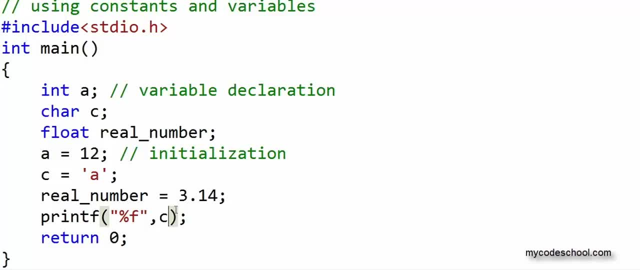 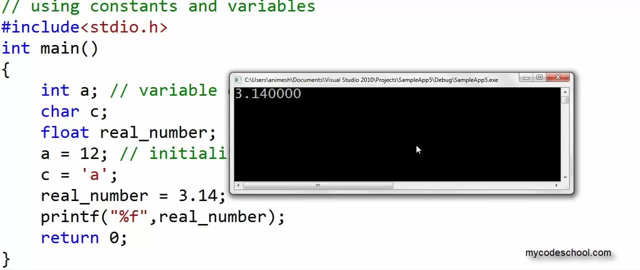 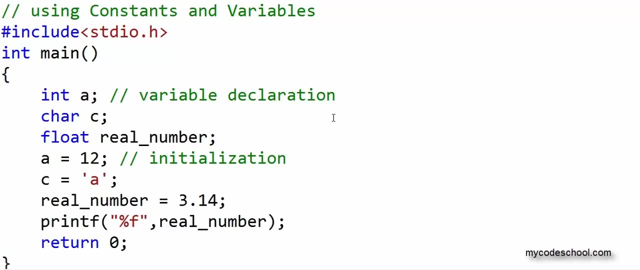 in this variable we need to say percent f And then we need to give the name of the variable as second argument. When I'm running this, as you can see, this real number is getting printed. Okay, so with this much, we understand how to store basic primitive data in variables. In our next lesson,